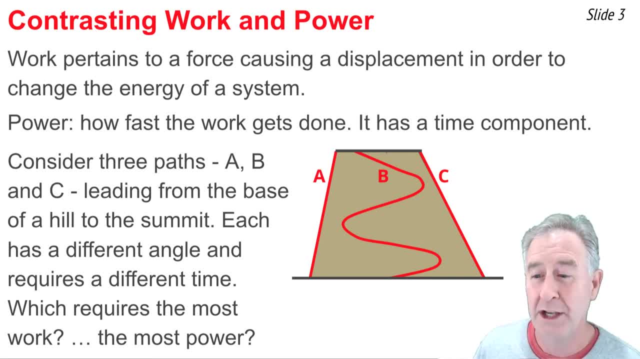 the base of the summit in the least amount of time and in the least amount of distance. But path B is the path that has many cutbacks leading from the base to the summit And it would require the most amount of time due to its greatest distance. Path C is somewhere. 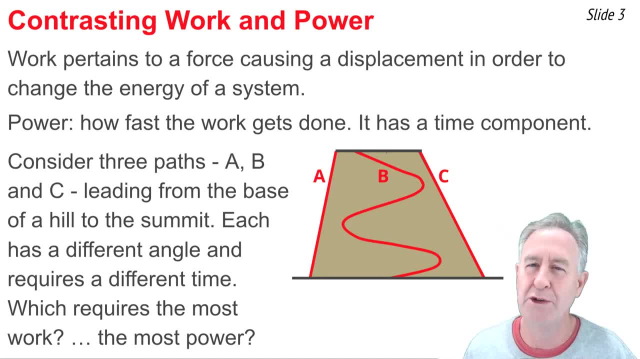 in between. Now, when we think about the question of which requires the most amount of work, we have to think in terms of energy. All three paths lead from the potential energy at the base to the power, The potential energy, at the summit, And as such, they each require or each change the 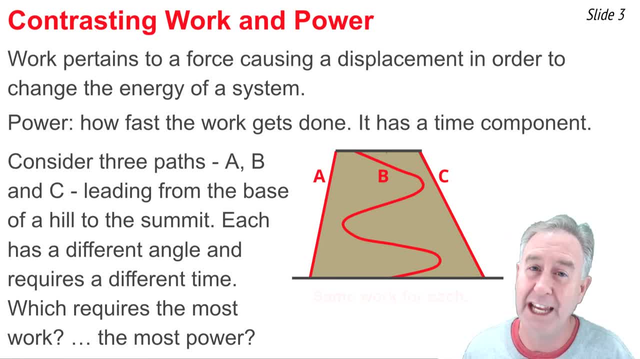 energy of the object by the same amount, And so they each require the same amount of work. But path A is done in the least amount of time And path C in the most amount of time. So A is the path that requires the greatest power, because it's the one that's done fastest. 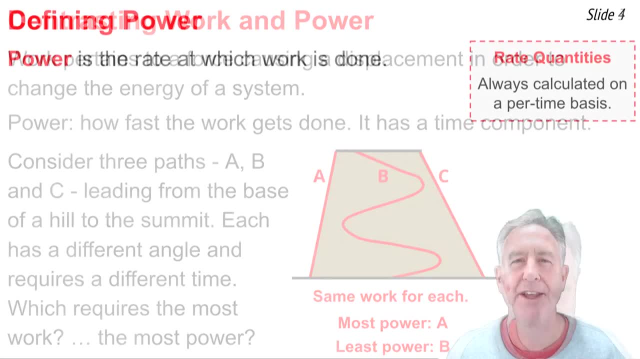 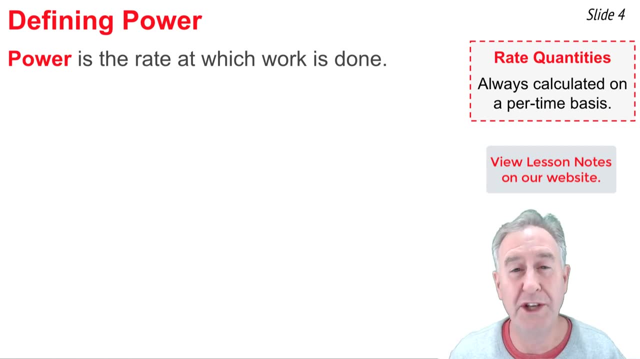 And path B has the least power. The textbook definition of power is the rate at which work is done. In physics, rate quantities are quite popular And they're always calculated on a per time basis. So when we say power is the rate at which work is done, what we mean is that power. 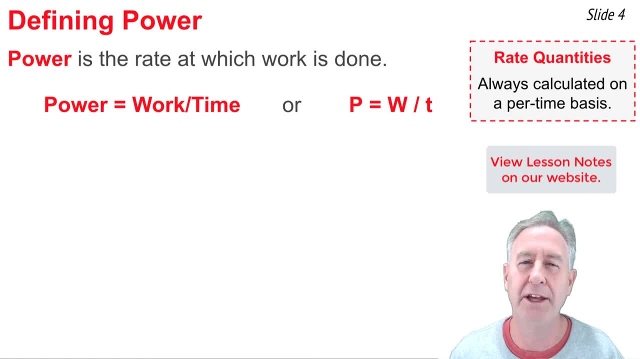 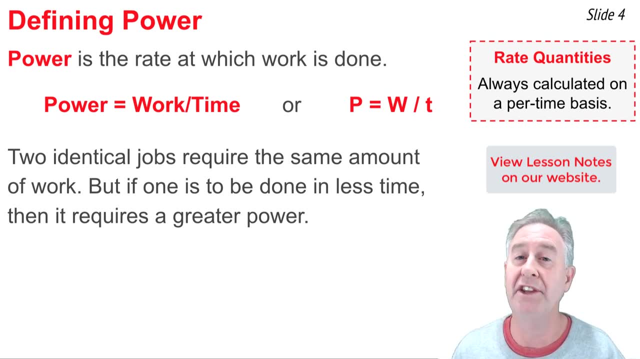 equal work per time, Or, in symbol form, P equal W per T. You could have two identical jobs, each requiring the same amount of work, But the one that is done in the least amount of time is the one that has the smallest denominator And, as such, it would be the one with the greatest. 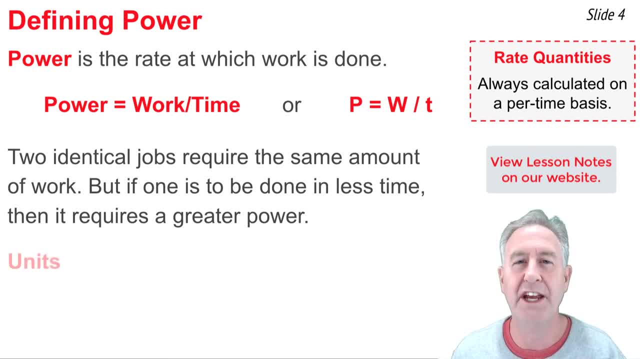 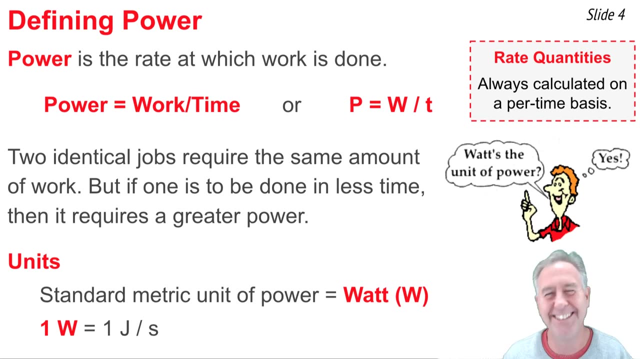 power, And this is the one that's done at the greatest rate. The standard metric unit of power is the Watt, abbreviated W, where 1 Watt is equal to 1 Joule per second. So if anybody ever asked you what's the unit of power, You would say yes. 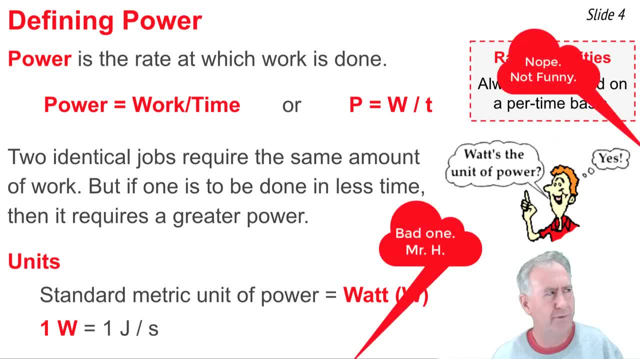 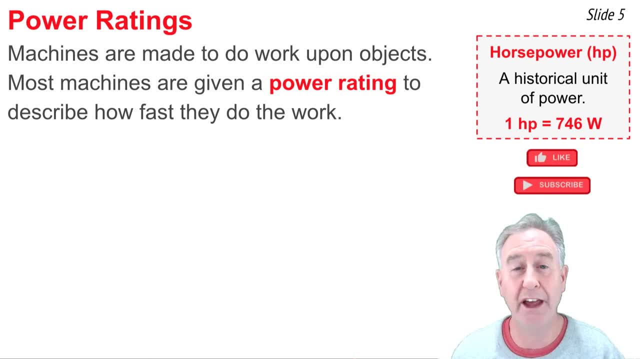 Come on, that was funny. That was like a dad joke. Machines are made to do work upon objects, But machines don't have a work rating. Instead, they have what's called a power rating. Power ratings describe how fast that machine does its work. 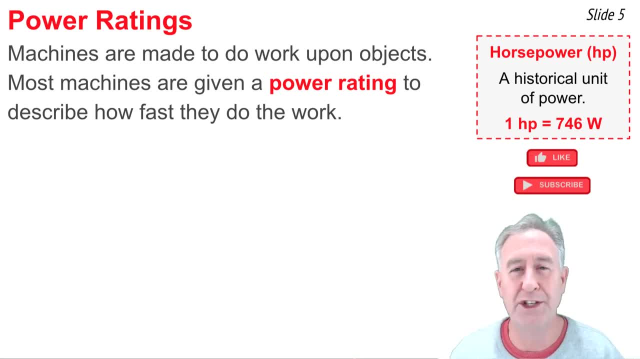 and they're usually listed in the unit horsepower. Horsepower is not a metric unit, but a more historical unit that dates back to the days in which we used to use horses to power most machines. One horsepower is equal to 746 watts To illustrate the idea of a power rating. 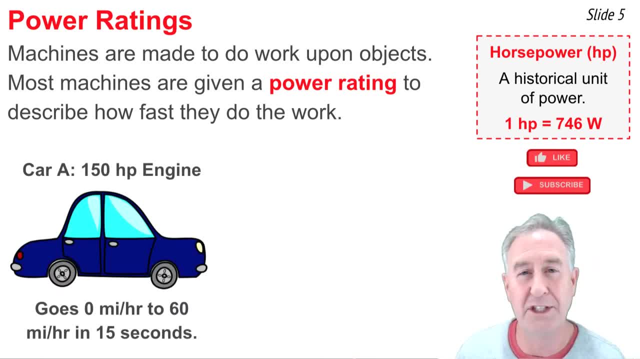 let's consider two car engines. This is car A, with its 150 horsepower engine, and with that engine it can go from zero to 60 miles per hour in 15 seconds. But this is car B. Car B has a 750 horsepower engine. 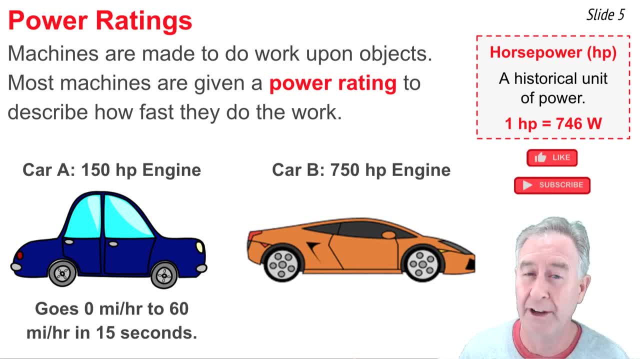 750 horsepower is five times the horsepower of car A and as such, it can do its work at a five times greater rate, which would mean that it could go from zero to 60 miles per hour in one fifth of the time- in three seconds. 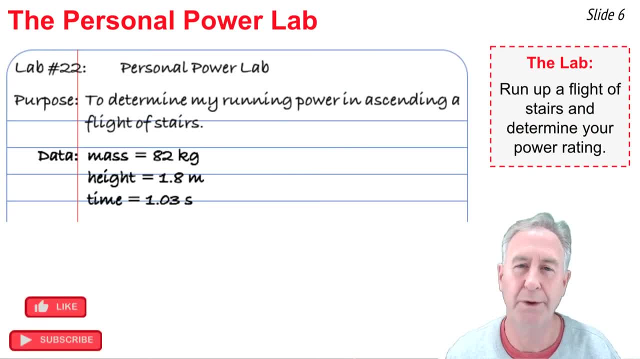 A common lab in a physics course is that personal power lab, or sometimes called the staircase lab. In the lab, students run up a flight of stairs, usually at constant speed and as fast as possible, in order to determine their power rating. Here's a lab notebook entry for one such lab. 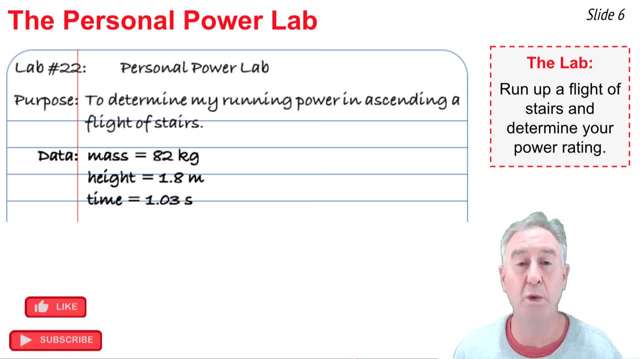 The mass of the person is 82 kilograms. The person climbs 1.8 meters high and does it in a time of 1.03 seconds. To determine the power, we need to first determine the force that the person applies to lift themselves up. 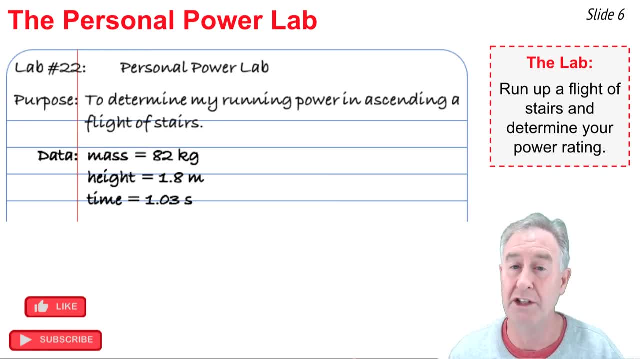 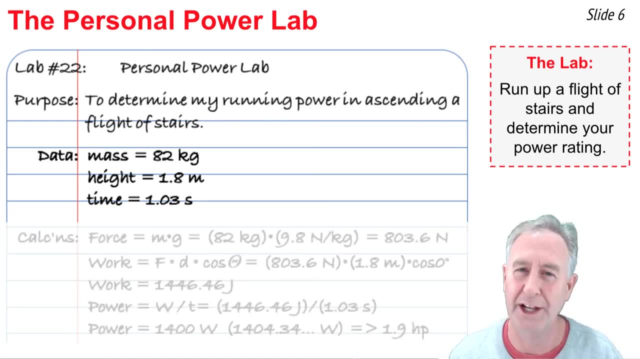 We'll assume, at a constant speed. and then we need to use force and displacement in order to determine the work and finally, the work with the time, in order to determine the power. The calculations go like this: For the force, we'll say the upward force. 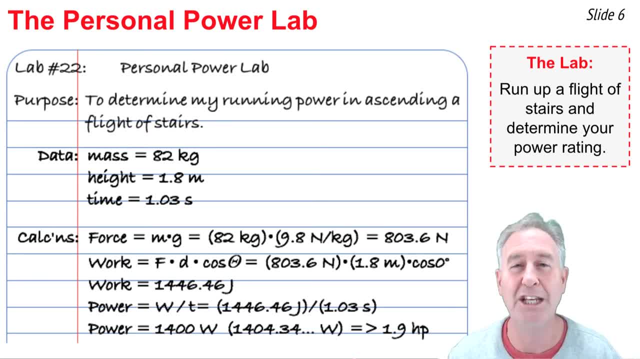 is equivalent to the force of gravity, which is m times g, 82 kilograms times 9.8 newtons per kilogram, which gives us a value of 803.6 newtons for the force. Now I can calculate the work. 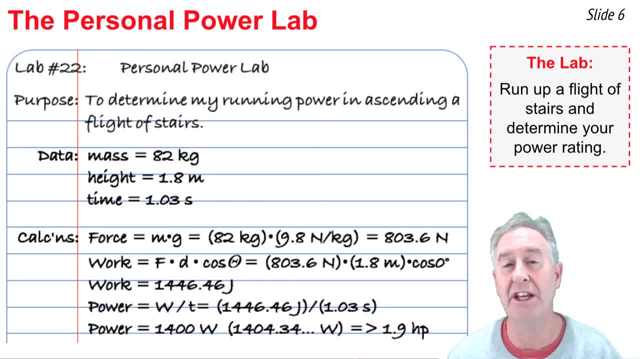 The work is the force times the displacement times, the cosine of the angle between the force and the displacement. So we will go 803.6 newtons times 1.8 meters, times the cosine of zero degrees, and we get 1,446, and some change joules. 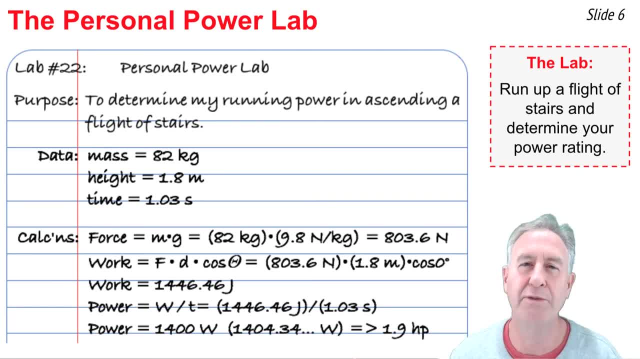 Now we're ready to calculate the power. We'll go 1,446.46 joules divided by the 1.03 seconds and we get a power of 1,404, and some change watts or rounded to 2 significant. 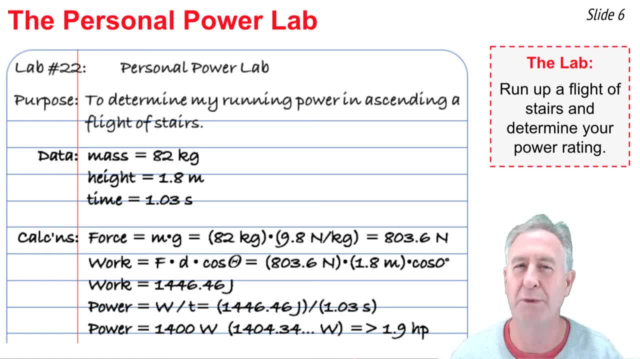 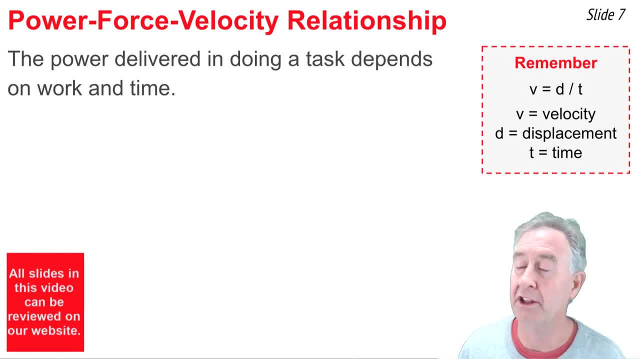 digits, about 1400 watts. This is equivalent to 1.9 horsepower. The power delivered in doing a task depends upon work and time. We've expressed the relationship as power equal work divided by time. If we presume that the force and the 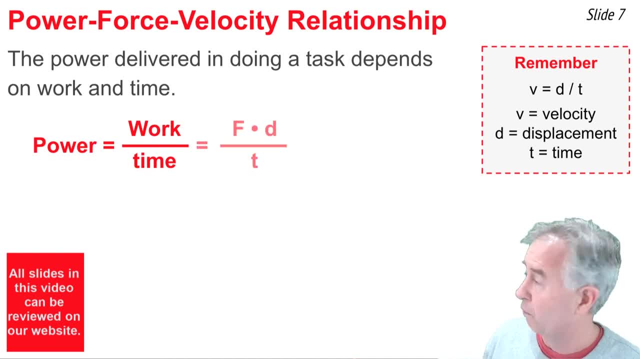 displacement are in the same direction. we could call the numerator force times displacement. So power equal force times displacement divided by time. Now the d in the numerator and the t in the denominator might be recognized as the velocity. So the power is equal to. 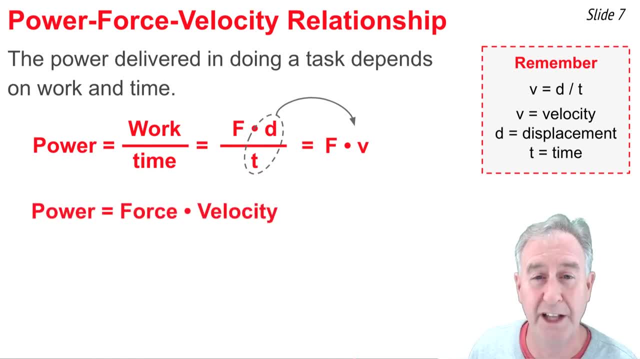 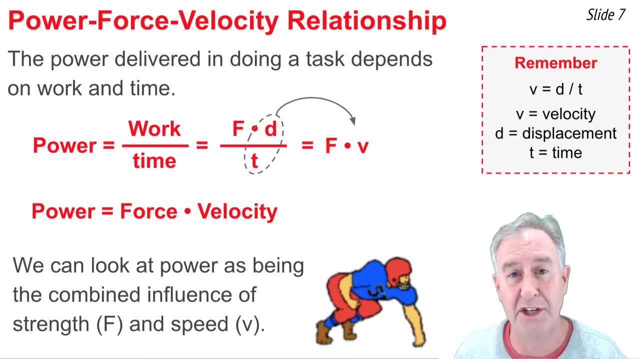 the F times the V, or power equal force times velocity. So when it comes to a power rating, we can begin to think of it as being the combined influence of force and velocity. If we apply a power rating to a football player, we might say that the lineman with the greatest power 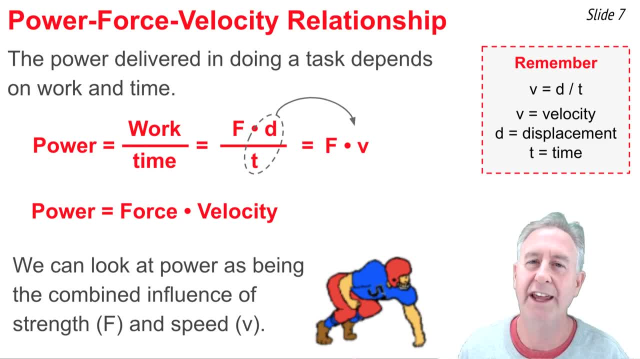 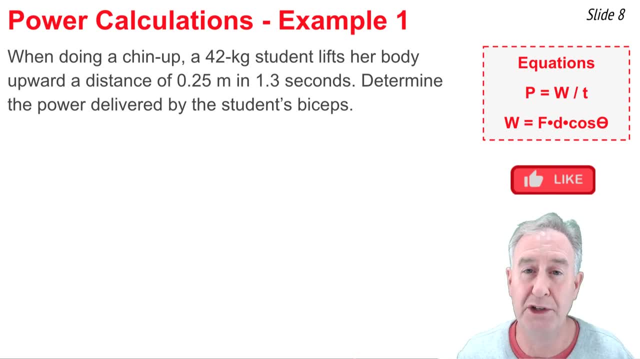 is the one that has the greatest strength, applies the greatest force and the greatest speed. It's common in a physics course to have to solve a problem, A problem in which you analyze a physical situation to determine the power rating. A problem like this one about a student doing a chin-up with a mass of 42 kilograms lifting. 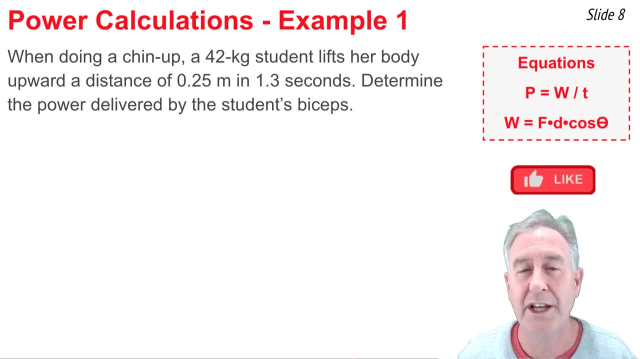 herself upward 0.25 meters in 1.3 seconds. Now, in this case, we're going to begin by listing what we know. We know the mass, the displacement, the time and since it's an upward force to cause an upward displacement, the angle theta is equal to 0 degrees. I'm 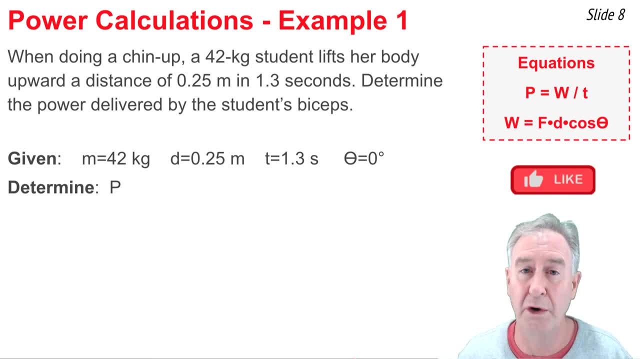 looking for the power, My first step would be to determine the force. If this person lifts themselves upward at constant speed, then the up force has got to be equal to the down force. So we can safely say that the up force is equal to the force of gravity. 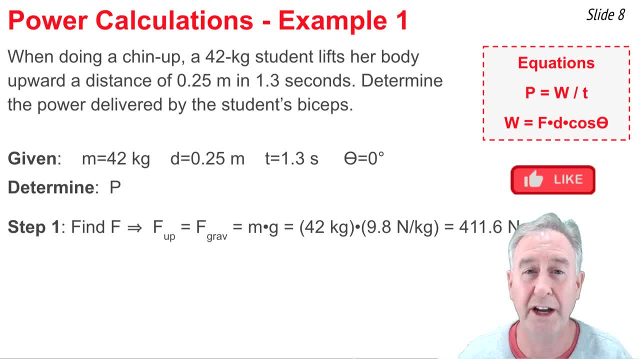 M times g, 42 newtons times 9.8 newtons per kilogram, and that's 411.6 newtons. Now I have to determine the work done in lifting herself 0.25 meters. So I'm going to take the force. 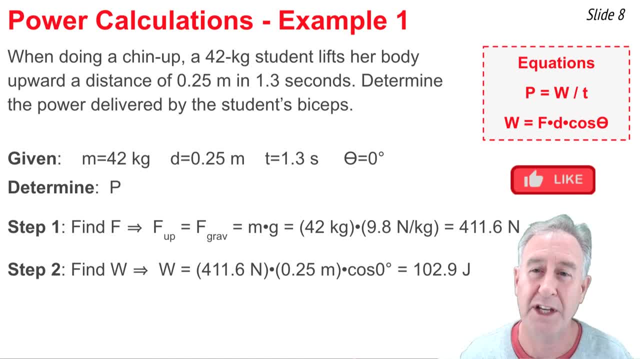 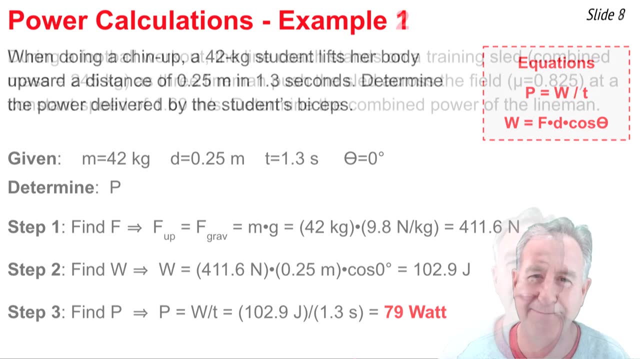 multiply by 0.25 meters and multiply by the cosine of 0 degrees, And I get 102.9 joules of work. Now I'm going to calculate the power by dividing the work by the time. That would be 102.9 divided by 1.3 seconds And I get approximately 79 watts. 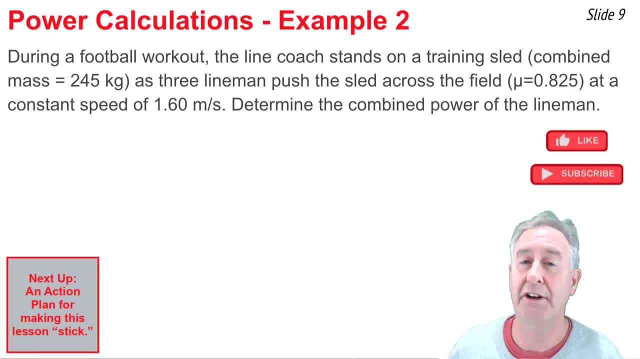 Our second and final example involves a horizontal motion During a football workout. the line coach stands on a training sled with a combined mass of 245 kilograms, as three linemen push the sled across the ground with a constant speed of 1.60 meters per second. The coefficient 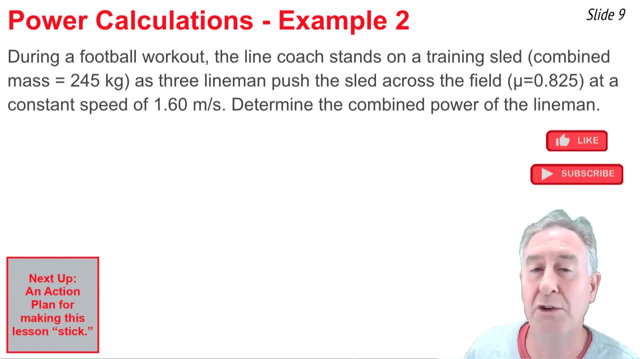 of friction mu between the sled and the coach is 0.2.. 0.3 seconds in the ground is 0.825.. We want to know the power delivered by the lineman. So, as always, we're going to begin by listing what we know. We know the m, we know the mu, we know the velocity. 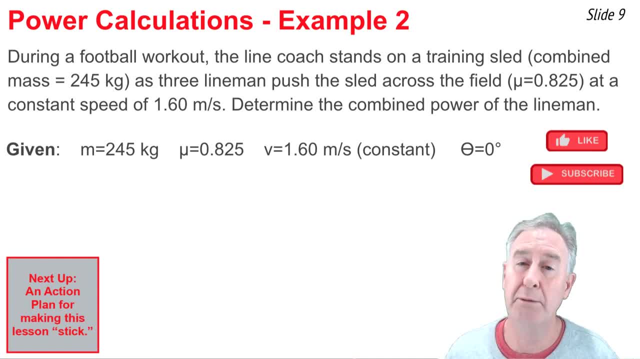 of the sled. and we know that the angle between the force the lineman apply and the direction that the sled moves is zero degrees. So now we can calculate the power. We'll begin by determining the force that the lineman apply to the training sled. That force would be equal to the force of 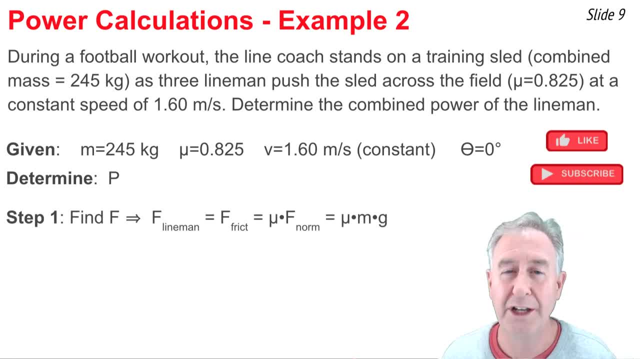 friction, since we have a constant speed motion. So the force of friction is always equal to mu times F norm and on horizontal ground that would be mu times the weight of the object, mu times mg. So we can substitute 0.825 for mu and 245 kilograms for the mass and 9.8 newtons per. 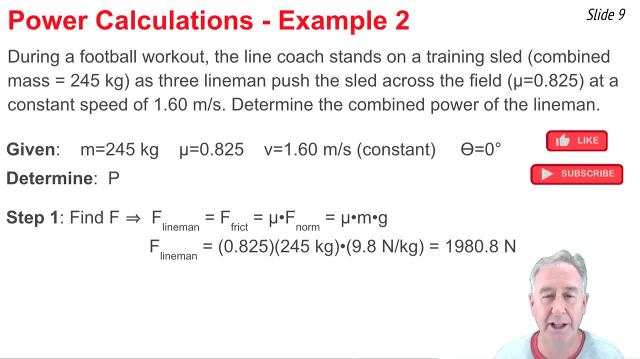 kilogram for g and we can solve for the force applied by the lineman. It's 1980.8 newtons. Now we know the force And we know the velocity. In an equation a few slides back said the power is equal to the force. 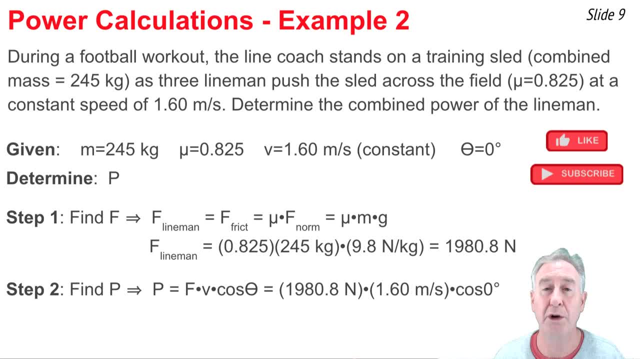 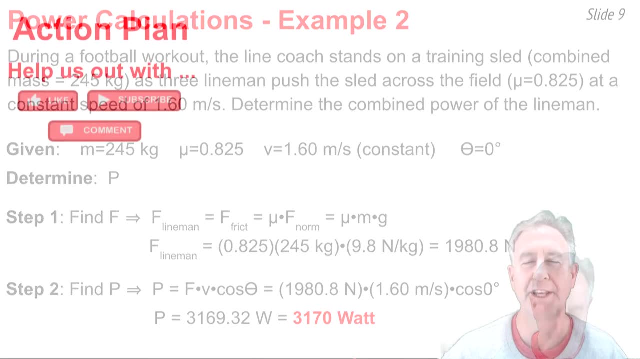 times the velocity. So we can take our force, multiply it by the 1.60 meters per second, and multiply it by the cosine of zero degrees and we end up getting 3169.32 watts, or rounding, we can say 3170 watts. It's at this time in every video that I like to help you out with an action. 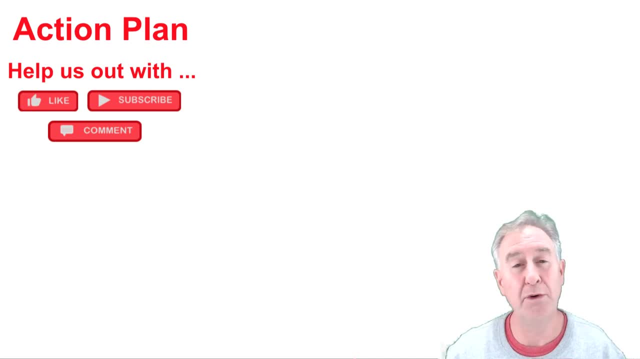 plan, a series of next steps for making the learning stick. But before I help you out, could you help us out by giving us a like, subscribing to the channel or leaving a question or comment in the comments section below? Now for your action plan. Here are 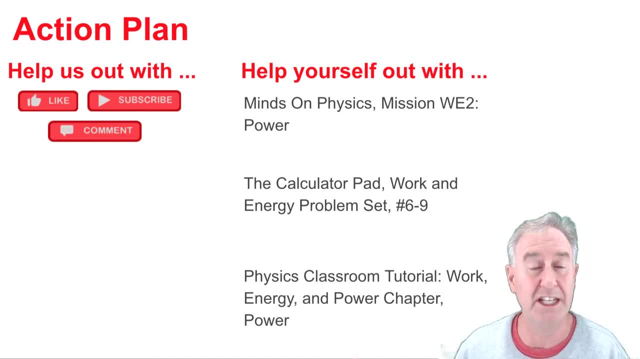 three resources that you can find on our website. We've left links to each of them in the description section of this video. You have a Minds on Physics mission a four problems from the calculator pad with problems, answers and solutions and a very understandable tutorial page. Whatever you do, 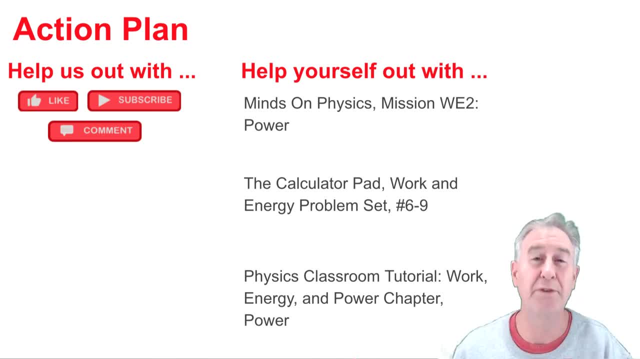 I wish you the best of luck. I'm Mr H and I thank you for watching.